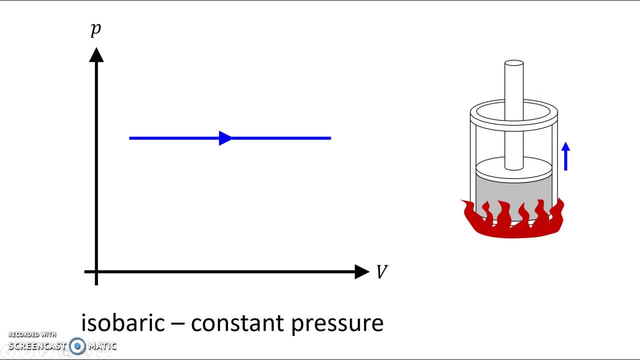 but you keep the pressure constant. The other way we could do this is by having an isobaric compression, So the volume will decrease. We're going from a bigger volume down to a smaller volume. How do we do that? We cool the gas and we let that piston slide down. 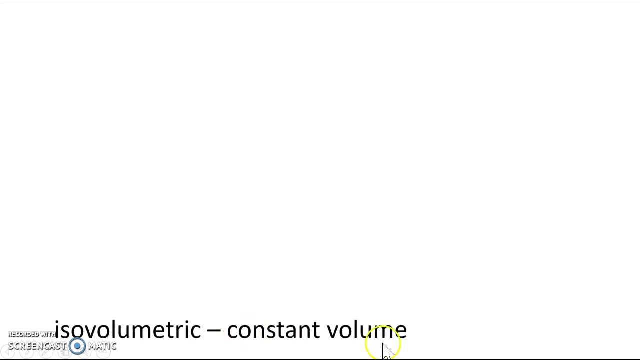 The next process is isovolumetric, which means constant volume. The way we make this happen is: well, we could have isovolumetric heating, And what we do is, if the volume doesn't increase, we don't move to the right on the x-axis. 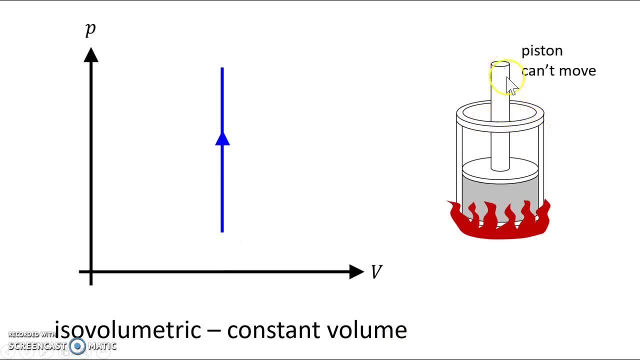 the volume doesn't decrease. we are going to fix that piston. We hold it in place so it can't move. When we add heat q, we raise the pressure. This is isovolumetric heating, But we could also have the line go down. 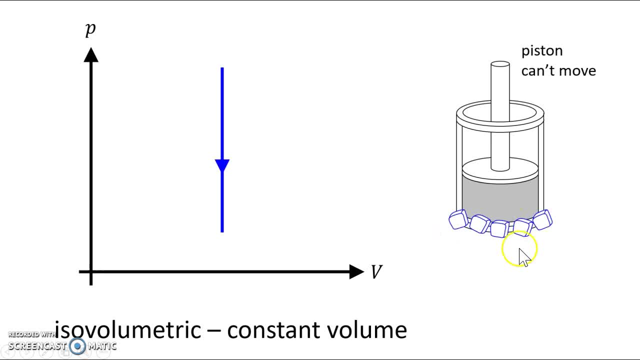 That would be isovolumetric cooling. The environment is at a cooler temperature than the system, the gas, so heat exits from the gas And as the heat goes out the piston can't move, so the pressure drops. The next graph is isothermal. 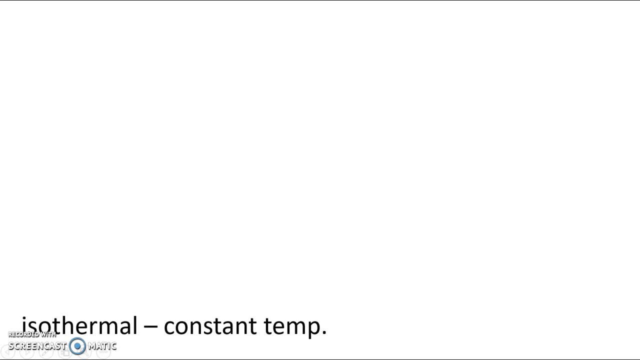 and this is one where the process has a constant temperature. Now isothermal graphs look like an inverse curve and I'm kind of exaggerating the shape here, but you'll see why in a second. Why would an isothermal process have an inverse shape? 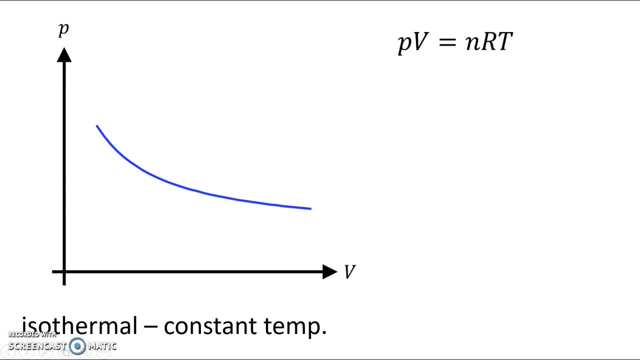 Well, we know that PV equals nRT. We're talking about an ideal gas as our system. This is the equation of state for an ideal gas. But if temperature is constant, well, R, the ideal gas constant, is also not going to change. 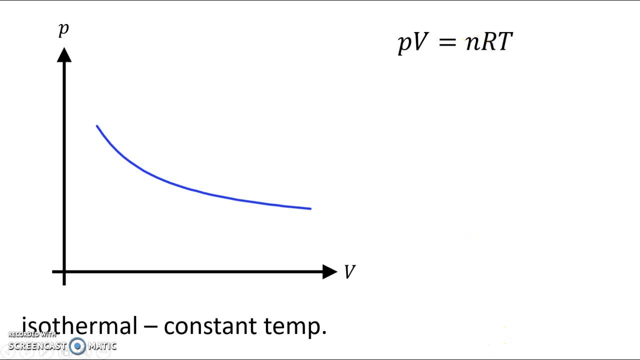 The number of moles is constant. Gas doesn't leak out of the piston or out of the chamber, so the whole right side is a constant. when temperature stays fixed, If we divide both sides by V, we get an inverse relationship. Now you can have this: 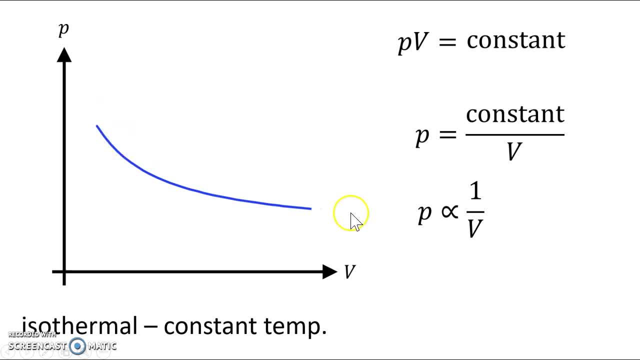 and you can have a temperature which would produce this type of graph. but you might also have a higher temperature And if you have a higher fixed temperature the graph is higher up. If you have a lower fixed temperature, the graph is a little bit lower. 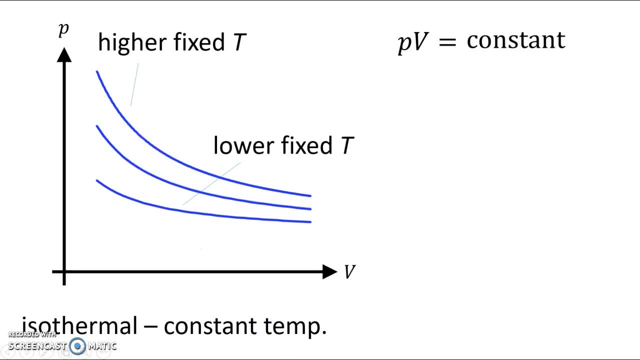 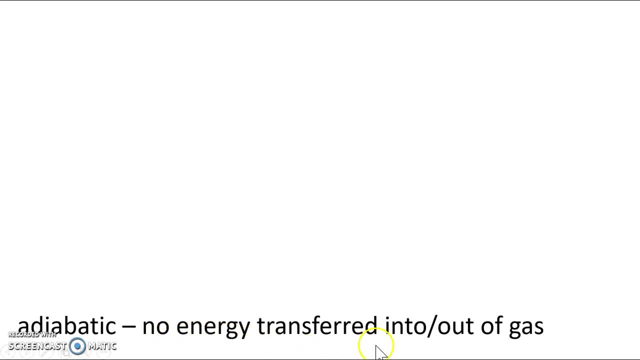 That's the difference between these different curves. The last process for us to look at is adiabatic. This is one where no energy is transferred into the gas or out of the gas. Now we have to be careful. What we mean by energy is heat energy. 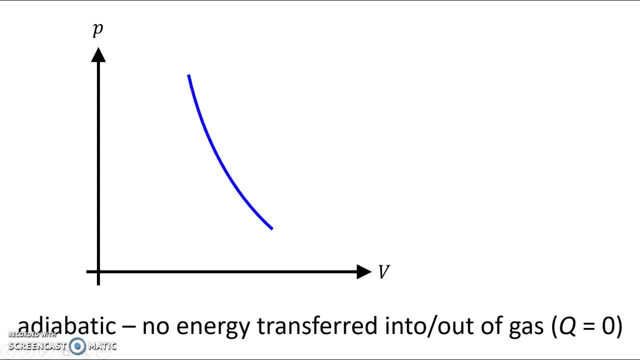 What does this look like on a graph? It's almost like an inverse curve, but it's much steeper. How do we make a process like this occur? Well, you could take your gas and you could just put it inside, you know. 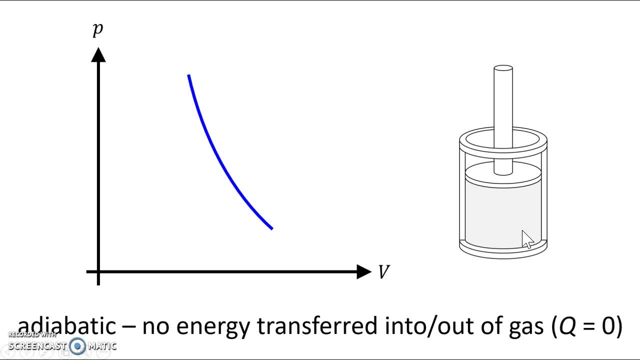 a thermoflask or whatever. the best thermos is something that's super insulating. Heat can't get in, Heat energy can't get out. But that's not very realistic. so what you might do instead, Ready You grab that piston. 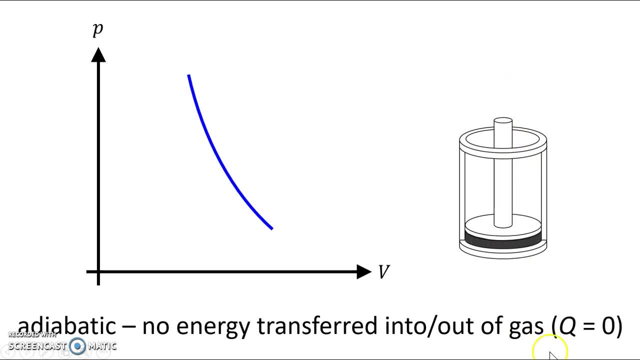 and you slam it down as fast as you can. What happens here is the gas heats up really fast, But you went so quickly. there's no time for that heat energy to get transferred out into the surrounding environment. That would be an adiabatic compression. 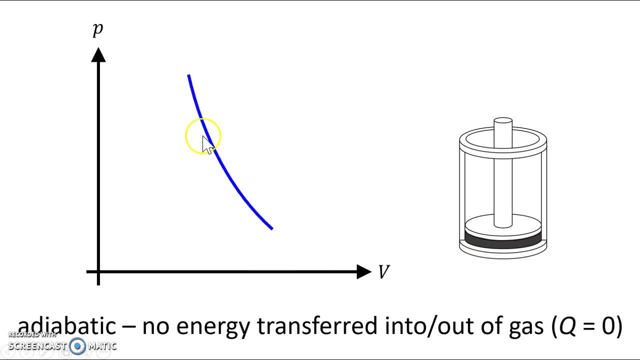 So which way would the line point? It would point to the left, decreasing the volume. Or you grab your piston and you pull it up really fast and the gas cools. but we haven't had any time for heat energy to transfer into the gas. 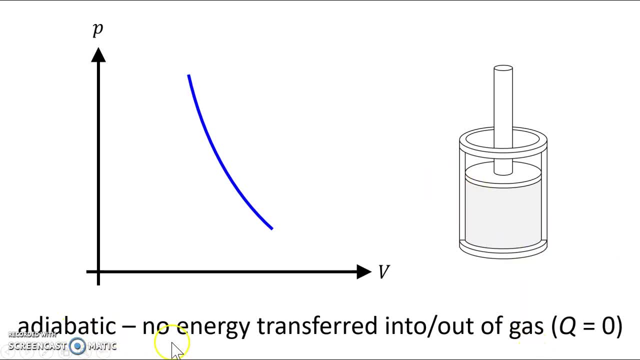 from the outside. That's why adiabatic processes typically have to be done very quickly. This is almost the opposite of an isothermal process. In isothermal processes, you don't want to go fast because you don't want the temperature to change. 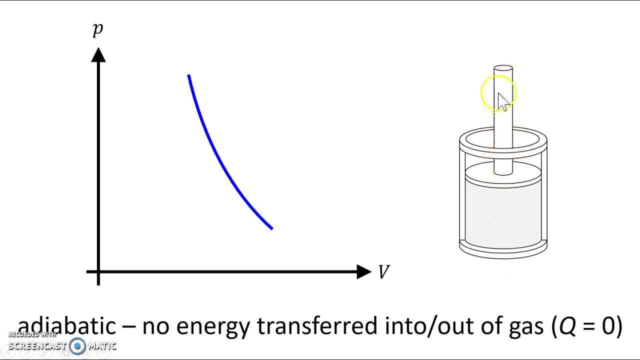 In isothermal processes you have to pull and push that thing very slowly so that the system, the gas, is always in thermal equilibrium with the surroundings. You don't want this getting too hot or getting too cold. There's one equation that I want to show you. 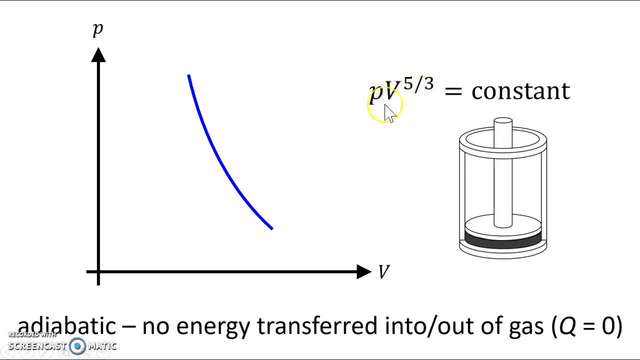 for adiabatic processes. It's almost the same equation for isothermal processes, But instead of PV equals a constant, it's P times V to the 5 thirds. So what happens here is there's a good reason why it's 5 thirds.